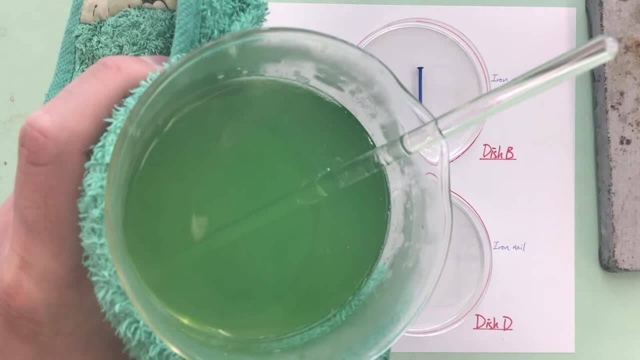 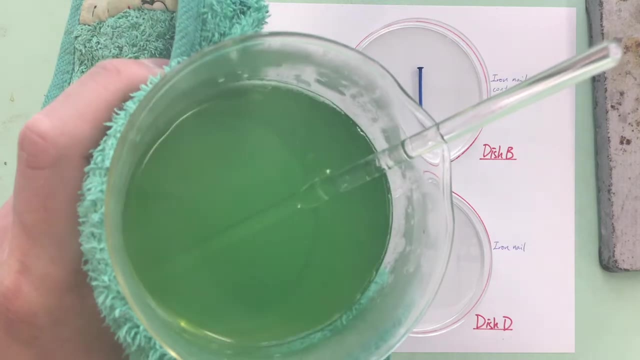 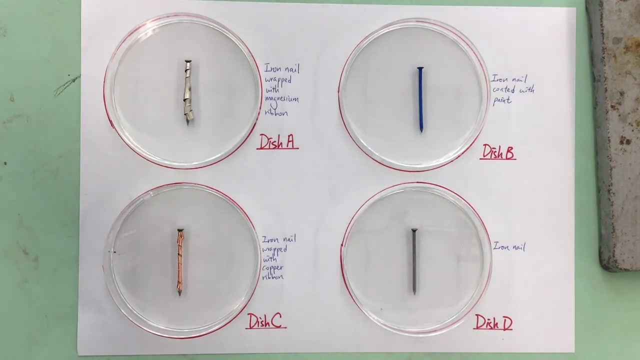 The gel is green in color due to the presence of hexacyanophery-3 ion. This gel is a liquid when it is warm And as it cools down it will coagulate to form a semi-solid. Pour the warm gel carefully into the petri dishes to cover the iron nails. 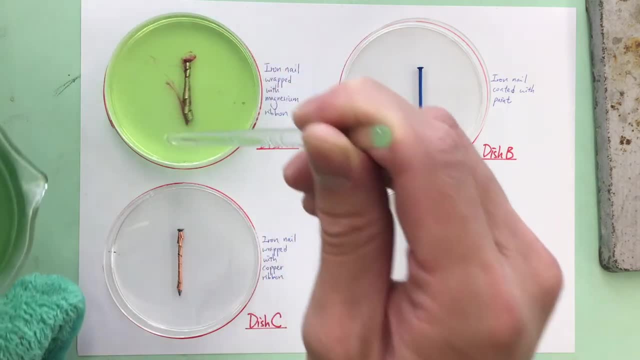 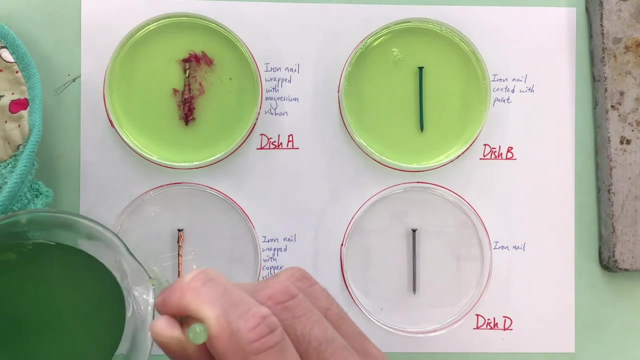 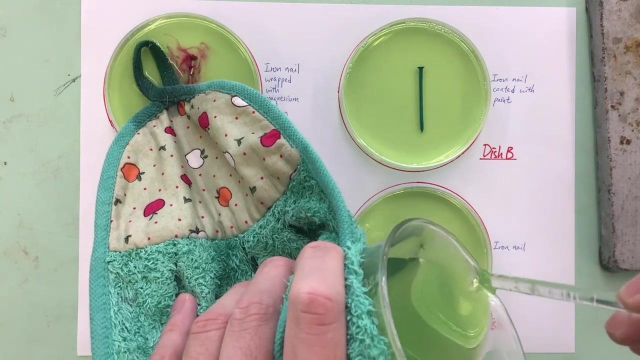 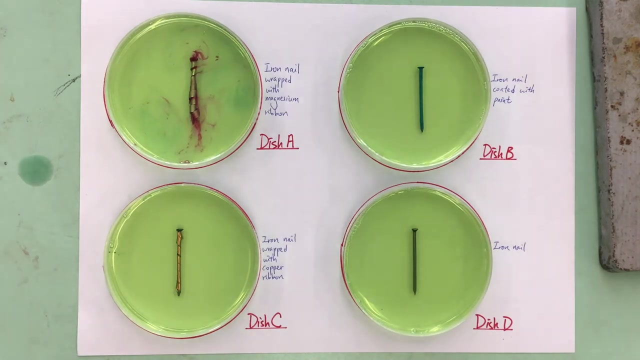 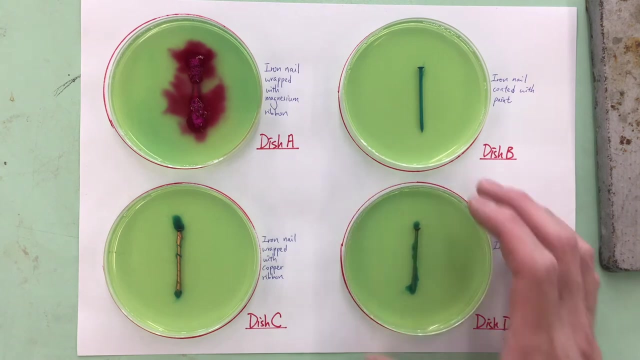 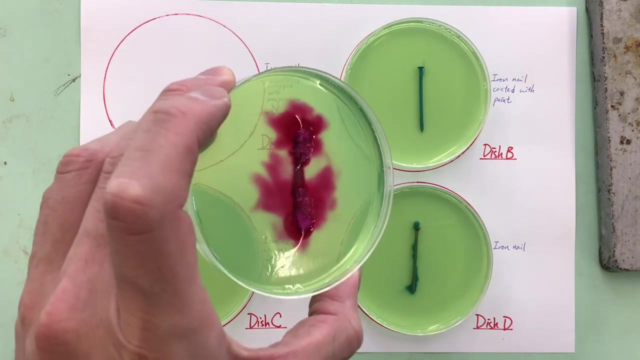 э Let the gel to cool down until it coagulates into a semi-solid. The gel has been cooled down into a semi-solid. Now we can perform our observation In dish. A red colour is observed, indicating the presence of hydroxide ion. 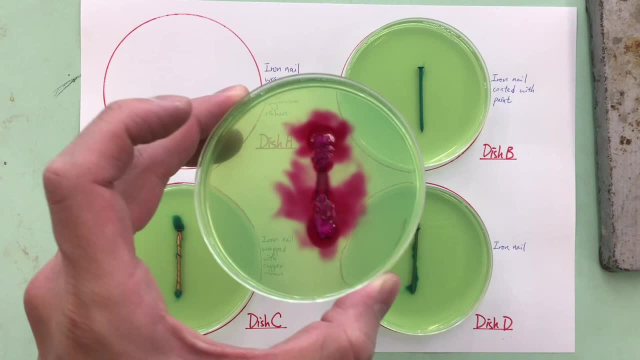 However, no blue colour is observed, indicating the absence of iron ion. These results suggest that no rusting had occurred. This is due to the sacrificial protection by the magnesium ribbon. since magnesium is more reactive than iron, Magnesium lose electron more readily than iron, and therefore preventing iron from losing. 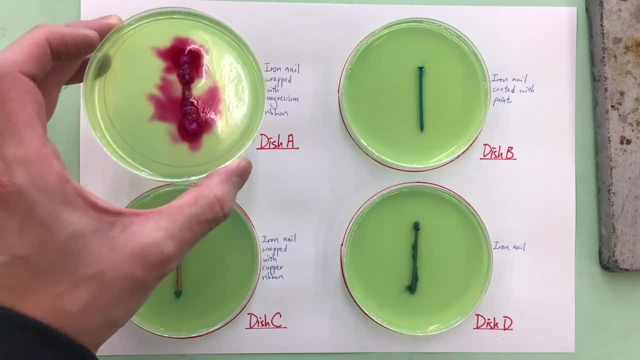 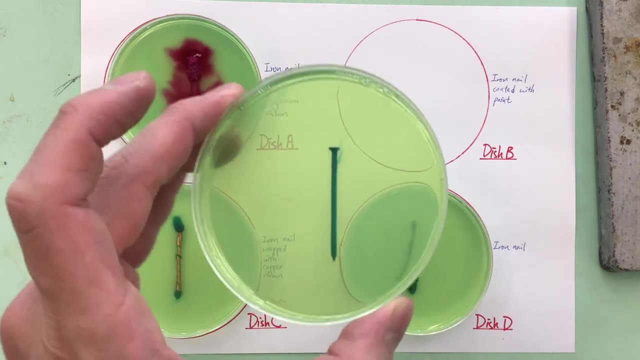 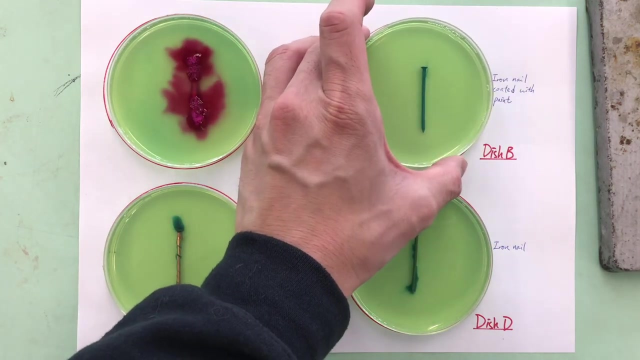 electron to form iron ion. In dish B, there is no observable change. This result suggests that rusting did not occur. The paint adds as a protective layer to prevent the iron from contacting with oxygen and water. In dish C, blue colour is observed. 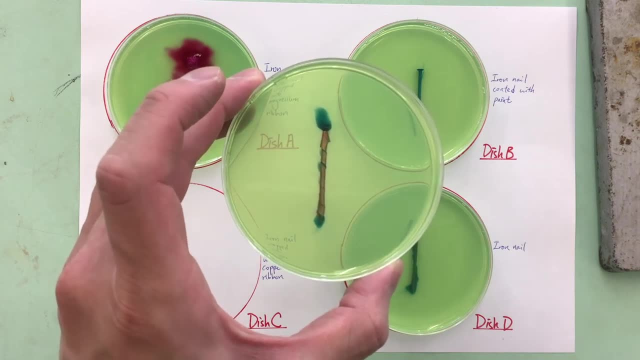 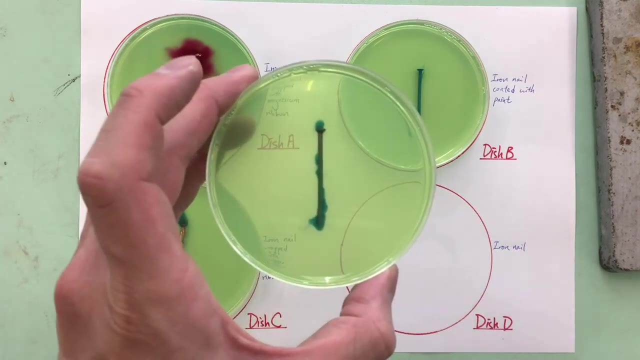 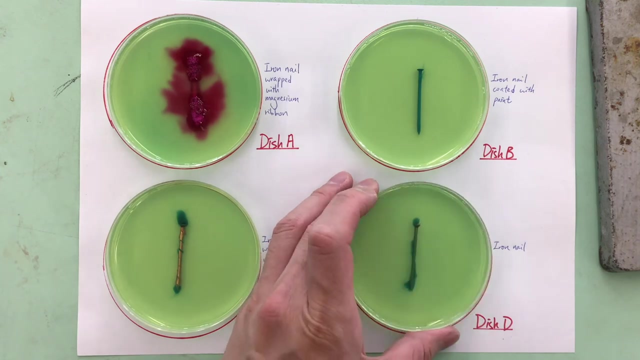 It indicates the presence of iron ion and it suggests that rusting had occurred. In dish D, blue colour is observed. It indicates the presence of iron ion. It suggests that rusting had occurred. In conclusion, rusting took place on the iron nails in dish C and dish D only.